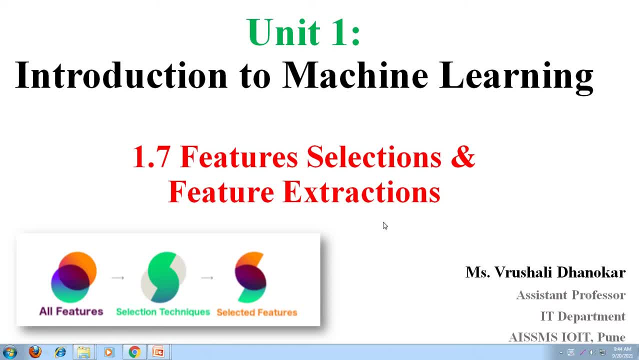 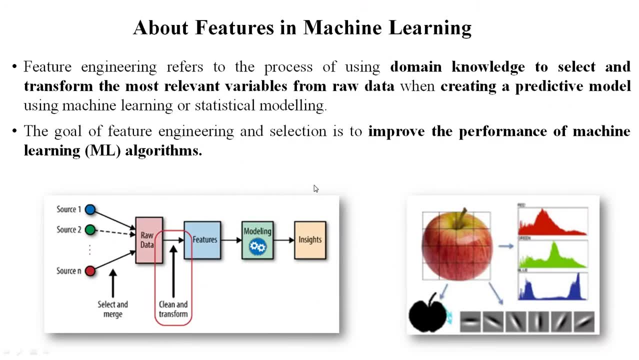 So I have mentioned the link of that videos in below description box. So let's see what is meant by feature selection and feature extraction. So we know that there are two types of engineering actually, that is, data engineering and feature engineering. So what is meant by data engineering? Data engineering means we have to perform different operations on data, like select the particular data, then insert, delete, 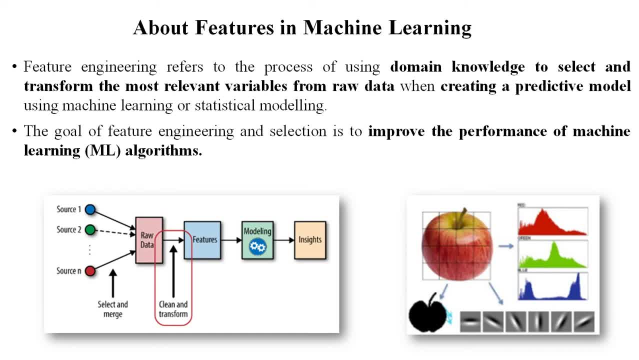 This kind of operation we will perform on the particular data set. This is called as data engineering, And on the other side there is again another thing That is called as feature engineering. So what is meant by feature engineering? Feature engineering is refers. it is a particular process to find out the relevant features of the particular data from your data set. 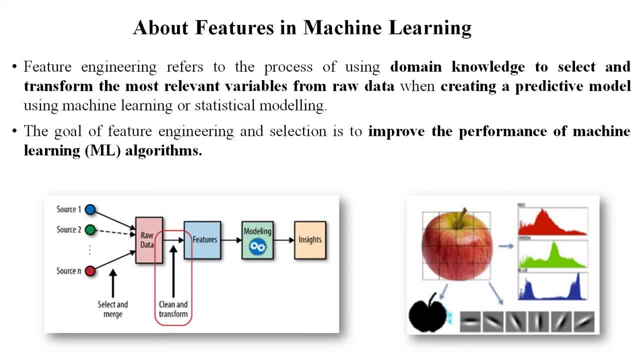 This concept is called as feature engineering. So feature engineering is a process of using domain knowledge to select and transform the most relevant features and these relevant features that will be used for creating the model. This concept is called as feature engineering. Now, what is meant by features? 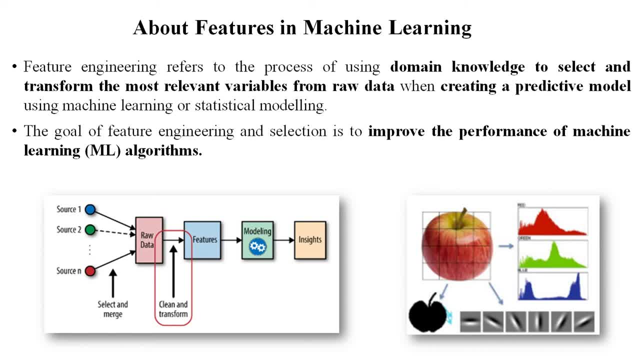 We can say. features means characteristics or specifications about the particular data. For example, there is a student data set, So their name, their roll number, their marks, This is called as features of students right. Another thing which is related to the images: 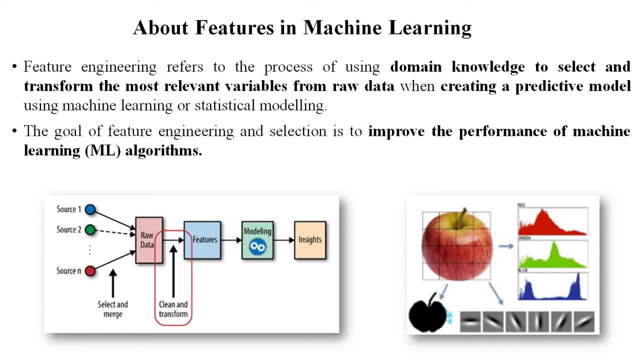 For example, this is the Apple image, So Apple having the particular shape and particular structure, they having the particular colors. So this is called a features of that particular data set. Now, what is meant by features? We can say features means characteristics or specifications about the particular data. 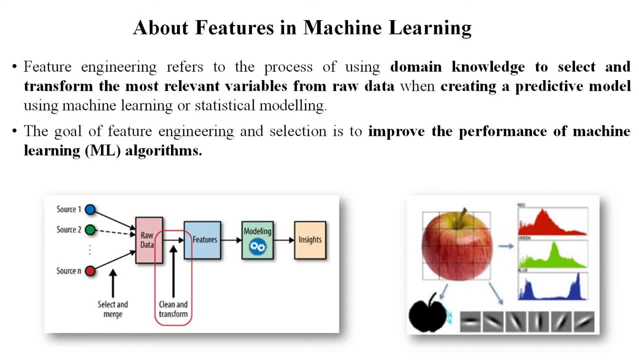 For example, there is a student data set, So their name, their roll number, their marks, This is called as features of students. right Another thing which is related to the images. For example, this is the Apple image, So Apple having the particular shape and particular structure, they having the particular colors. 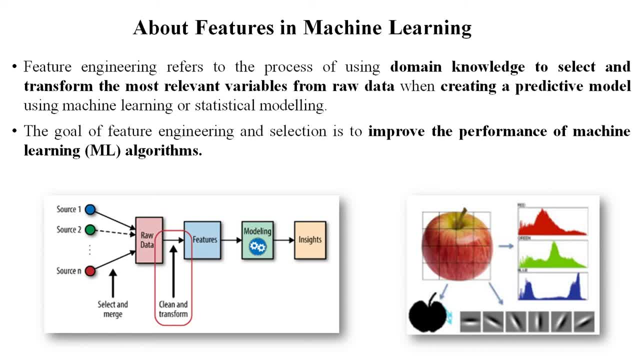 So this is called a features of that particular app, right, So this is the concept of features. Features means characteristics or specification, and to extract those features or to extract those relevant features for creating or for predicting a particular model, This concept is called as feature engineering. 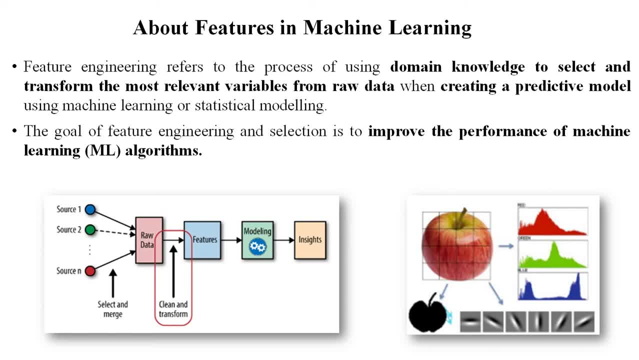 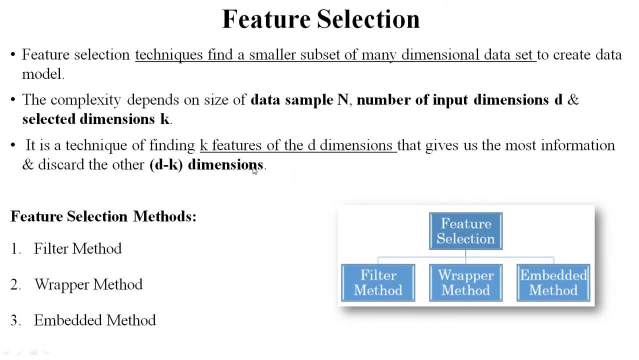 forth. So the goal of feature engineering and selection is to improve the performance of machine learning algorithms. Next Now, the next thing is feature selection. We have to perform two operations like feature selection and feature extraction. So first we will learn about feature selection. 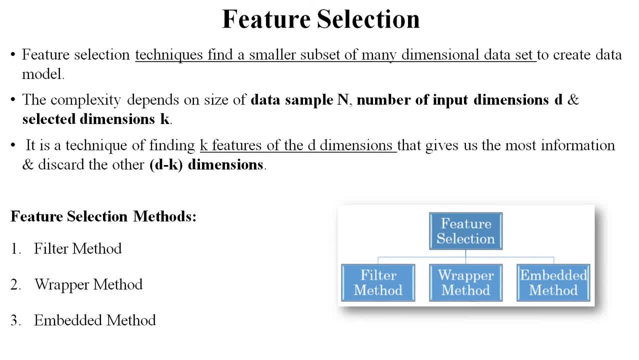 Now what is meant by feature selection? So feature selection is one kind of technique which is need to find a smaller subset of many dimensional data set. So first clear the concept about dimensions. Dimensions means sets of features. Just consider that. dimensions means the particular sets of features. 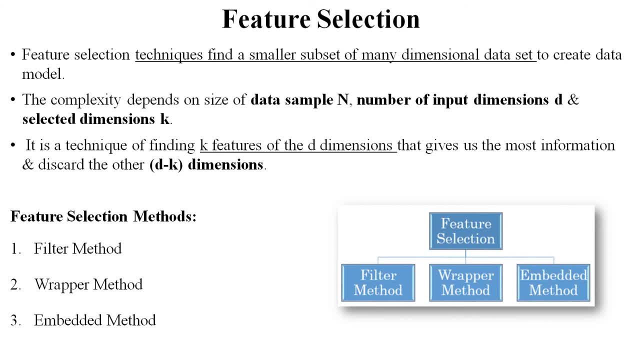 And find out the relevant features from this data set, which is called as feature selection. So there are in feature selection there are three methods like filter method, wrapper method and embedded method. Now in for feature selection, suppose just consider that there is n number of data samples. 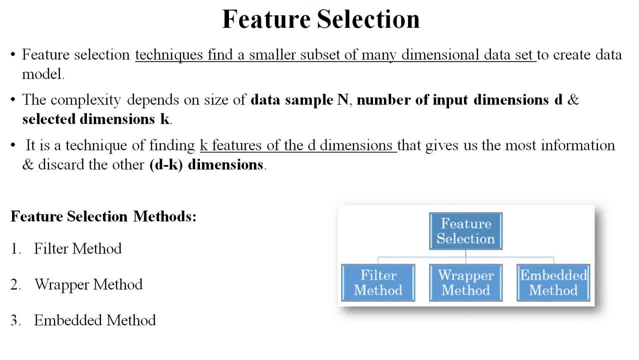 And there are d number of features of that particular data set. So you have to selected only k number of features from that d number of dimensions Means. suppose there are 10 number of features and you have to select only 5 number of features for creating the model. 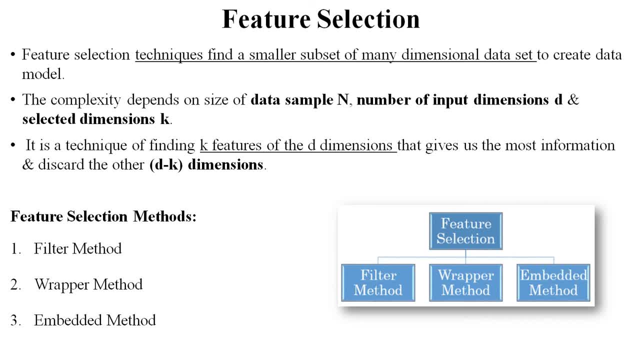 So 10 is called as dimensions, 5 is called as k dimensions means selected features And from that 10 minus 5 means remaining 5 features are there. So this 5 features are removed From that particular data set. 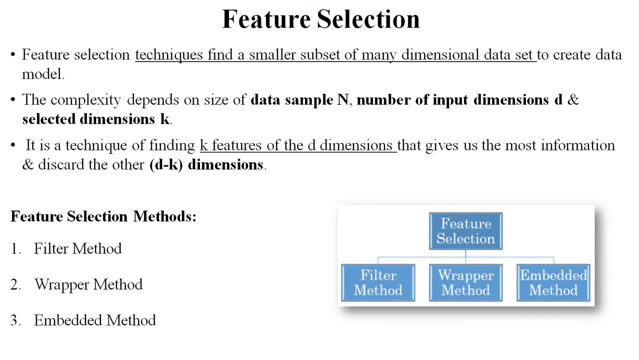 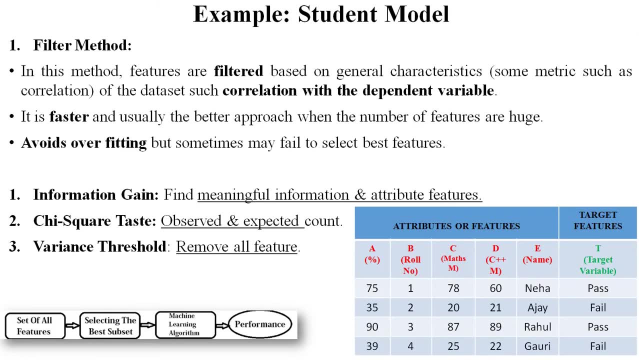 So this is the concept of feature selection. So let's see this. three methods of feature selection. next Now. the first method of feature selection is filter method. I will explain this concept by using student model. Okay, So let's see what is mean by filter method. 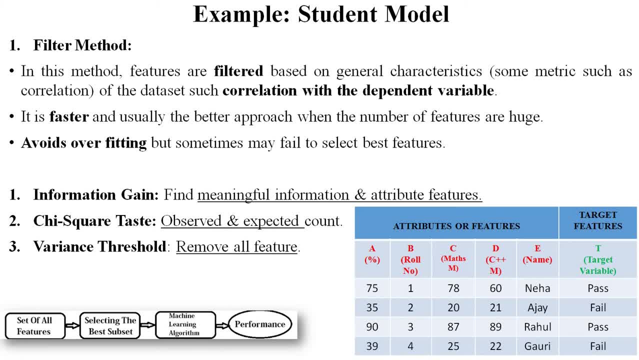 So in this filter method features are selected as per their characteristics or as per their correlation with dependent variable. Now see, in this diagram, in this table, there are total 5 features. Okay, This is called as attributes, or we can say features. that is percentage rule, number, maths marks, C++ marks and name of that particular students. 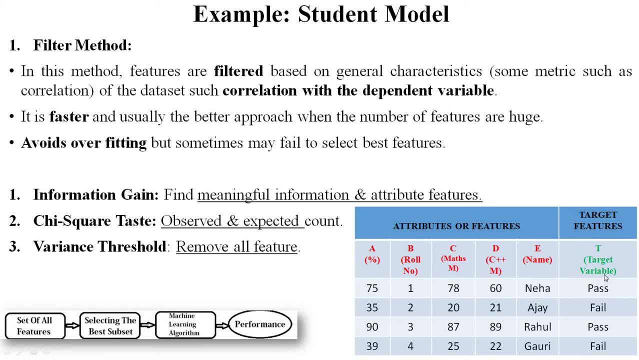 And our target feature is t, which is called as pass or fail Means. according to those features, you have to identify that the particular student is pass or fail. So let's see So by using filter method. we have to check the correlation with dependent variable. 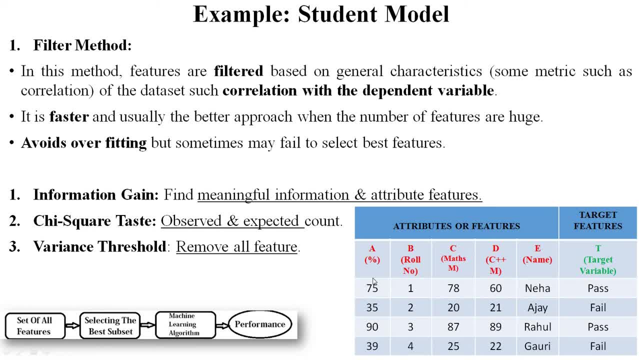 So let's see. So by using filter method, we have to check the correlation with dependent variable. So by using filter method, we have to check the correlation with dependent variable. See here the percentage. So according to the percentage, you can easily identify the particular student: is: pass or fail. 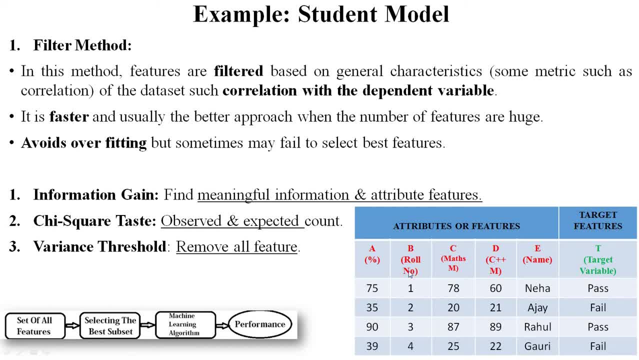 The particular student has 75%, then student is pass 35% that the particular student is fail. So the percentage is dependent variable on your target variable And this is the perfect feature Right Now. next one is role number. 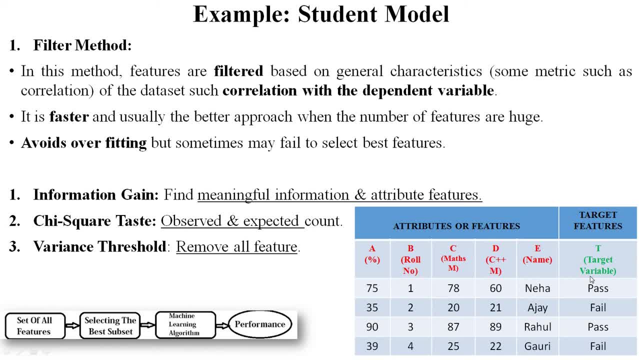 So is role number is a best feature for identify the particular student. is pass or fail? No, According to the role number, you can't identify that. So role number and name are the irrelevant features. according to the target features: Right. 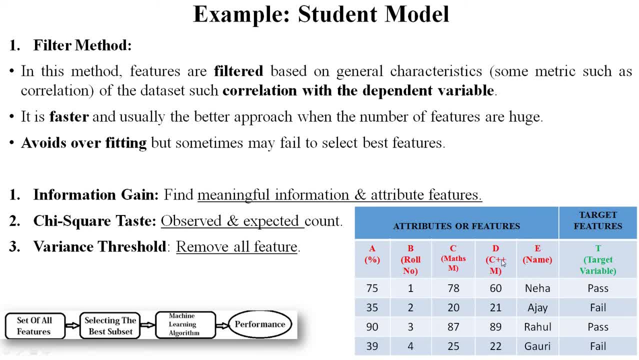 According to the role, number and name. you can't identify that Now maths and C++ Maths. So maths is also some kind of relevant features. But there is a percent column already there. Right, You have to calculate the percentage according to the maths. 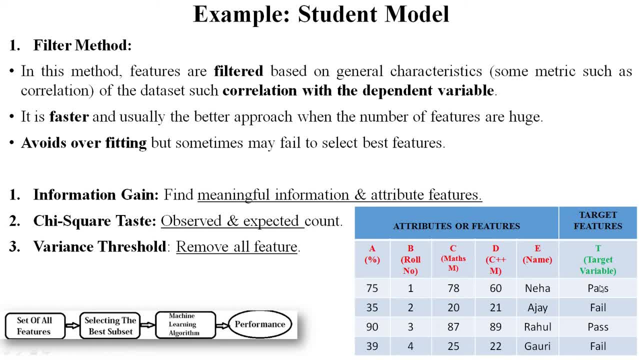 Right. So percentage is more relevant features. So filter method identify the more relevant features. That will be correlated and dependent on each other. Suppose I will change the 75 with 20 percentage, So the target variable pass is also change with fail. 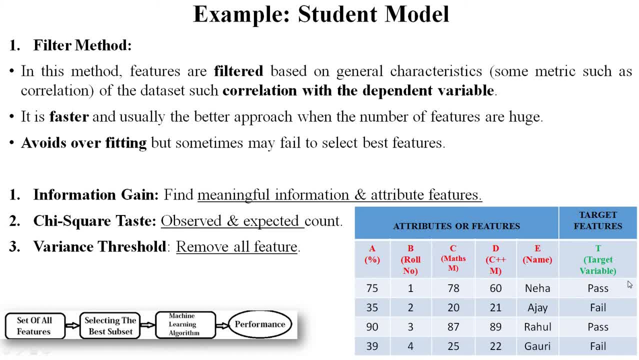 Right. So this is called as correlation or dependent variable. So the filter method is a faster method which is usually a better approach when number of features are huge, And it avoids the over fitting. concept means some errors are. it avoids the errors. 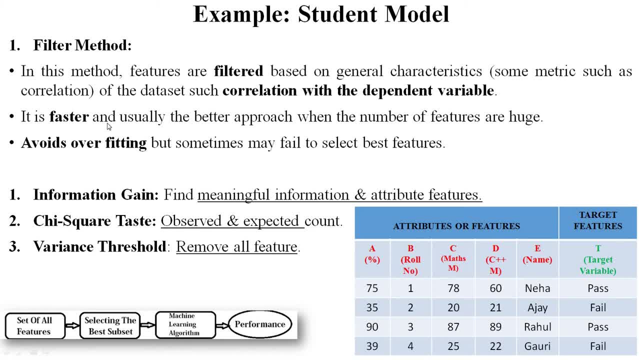 So may fail to select the best feature Right. So in filter method there is a information gain. Information gain means to find out a meaningful information And find out the best features from the given features: The feature which is related to your target feature. 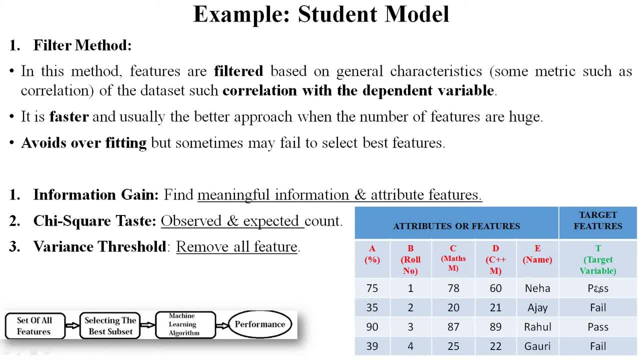 So here percentage is the best feature for calculating the student is pass or fail. So G square tells to observe an expected count of each and every features And variance threshold method remove all the other relevant features. So here, role, number, maths, C++, maths, name are the irrelevant features. 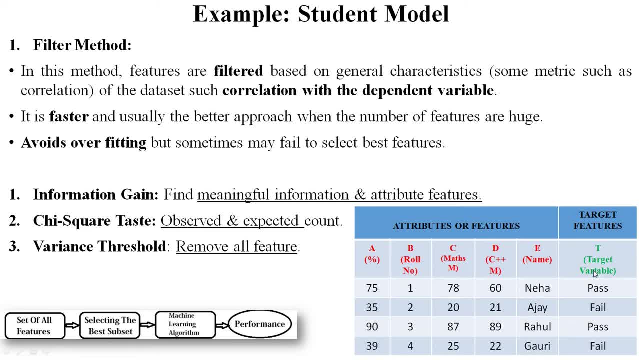 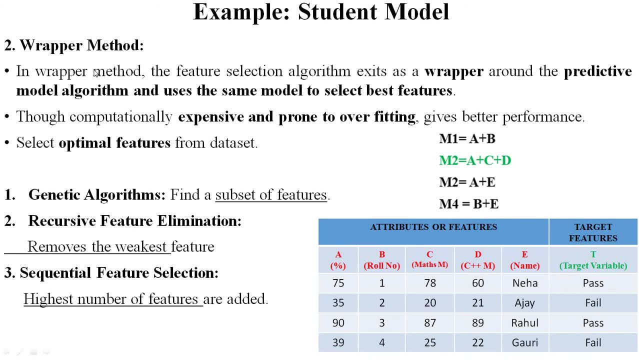 Right, That will be compared with the target features, Right? So this is a concept of filter method. In filter method that is dependent, variable or dependent features will be identified Next. Now the next method is wrapper method. So in wrapper method the feature selection algorithm is exist that wrap the sets of features. 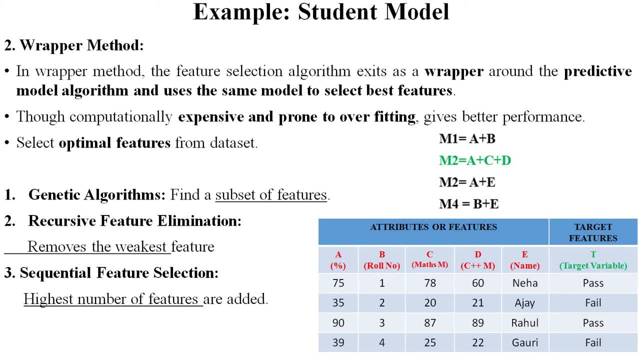 Okay, Wrap means combine the features. So as per their combining features, we have to generate a particular set of features, We have to generate a particular model. Now see here, in this same table, there are total 5 features, Right, 5 features of student. 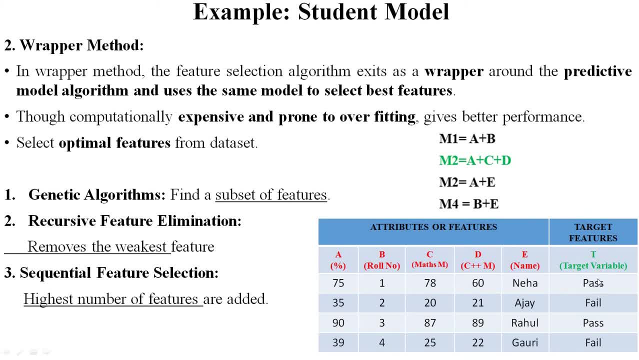 And our target feature is T, That is particular student is pass or fail. Now in wrapper method they generate a multiple models. See here the suppose. the first model is A plus B Means percentage and role number. According to this features and collecting this features, the M1 model is generated. 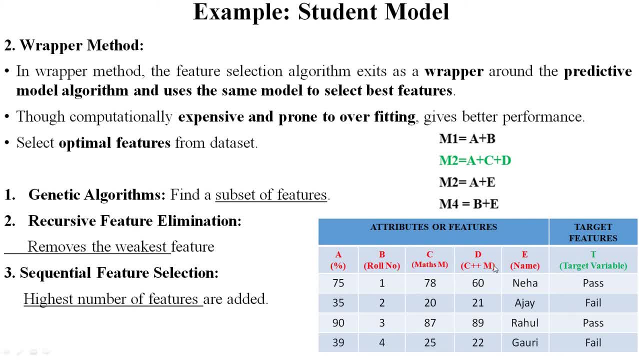 Now the next model is percentage and role number And the particular C++ marks. Okay, That is A, C and D Percentage match marks and C++ marks. So this collections of features, that is your next model, that is M2.. 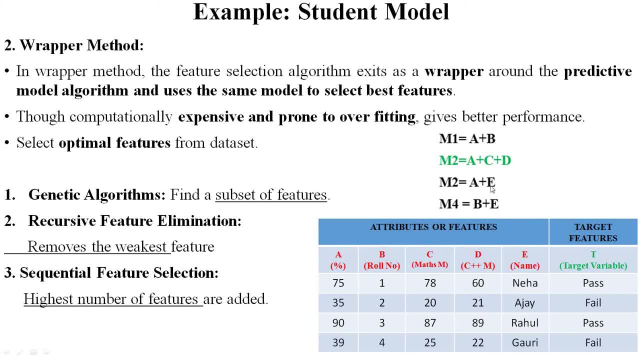 Now the next model is percentage and name. This is a wrapping features of your next model, that is M3.. Okay, Here is M3.. Then next one is a, B and E. That is role, number and name. This is another model. 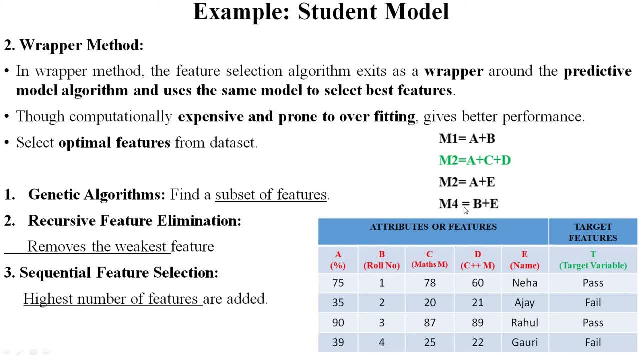 Okay, That is M4.. So there are four models are generated by wrapping a particular features. Now wrapper method: identify, which is the best model that identify the particular student is pass or fail. Now see here in this M3 model suppose: 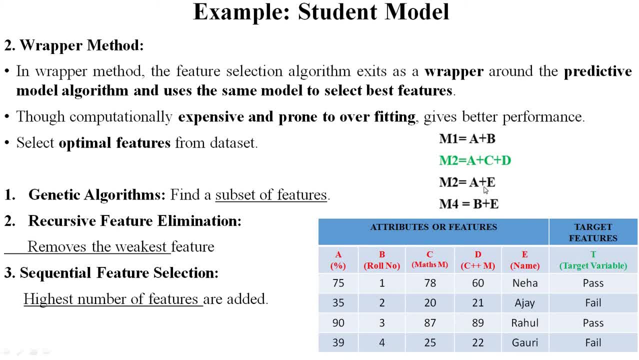 Role, number and name. This is the irrelevant model. This is not a best model to identify student pass or fail, Because there is only role, number and name. features are there Right Now. check with M2.. So in M2 that is percentage, then match marks and C++ marks. 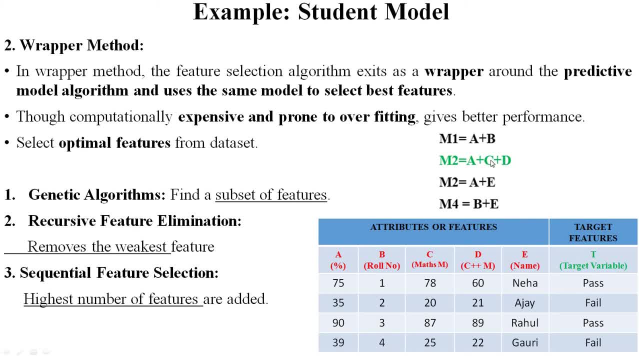 So these are the best wrapping features that will be generate a correct model and more accurate model to identify the particular student is pass or fail Right. So which is the model is best? that is, M2 model is best, Right. So this is called as predictive model or we can say wrapper method, to identify the wrapping features and to generate a model. 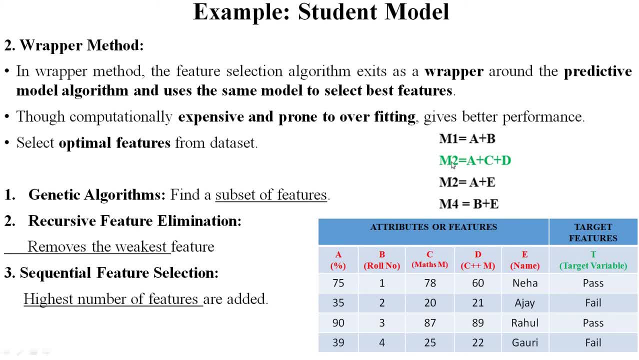 And this model test that the particular student is pass or fail. So this wrapping method is more expensive And prone to over fitting by giving a better performance Right. You have to select the optimal features from the data set. So in wrapper method there is some genetic algorithms are used to find out the subset of features. 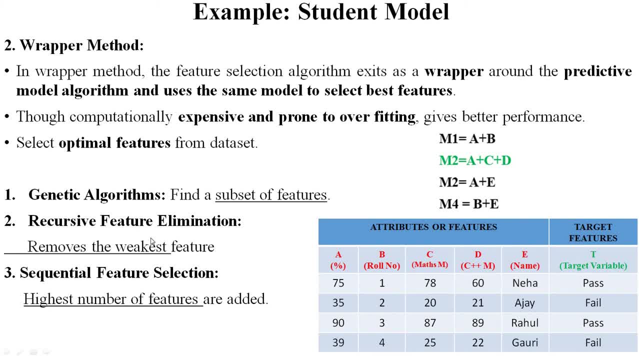 Right. Then recursive feature elimination. It remove all the weakest features, For example, role, number and name. These are the weakest features. So wrapper method: remove the weakest features and select only optimal best feature. Then sequential feature selection method Which is highest number of features. 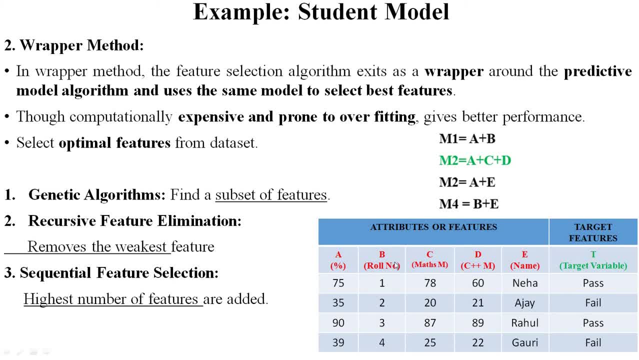 The highest number of features are added. If you add highest number of features in your model, then your model will be generate more accurate result Right. Or if you add either less number of features or relevant features in your model, then your model will be generate that approximate, not a correct one result. 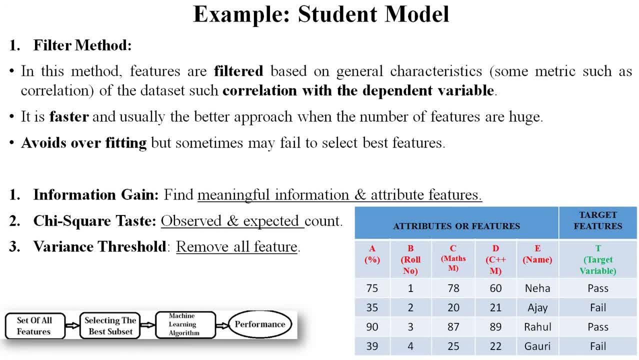 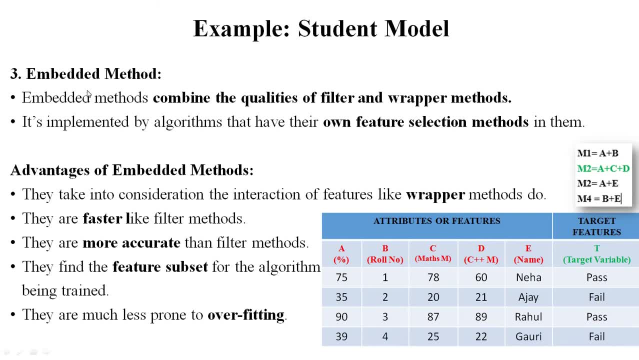 Right, So always add the best features in the particular model. Next Now, the next and last method of feature selection is embedded method. So embedded method is a combination of filter method and wrapper method. Right, They use the concept of both feature models. 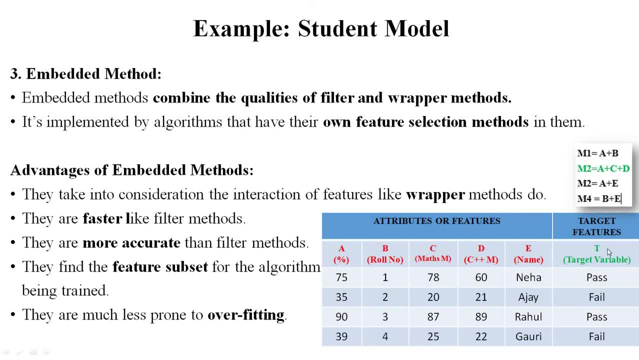 So see here, same table is there and again there are five features, that is, percentage role, number, maths marks, C++ marks and name. And this is your target variable. They, according to these features, you can identify the particular student is pass or fail. 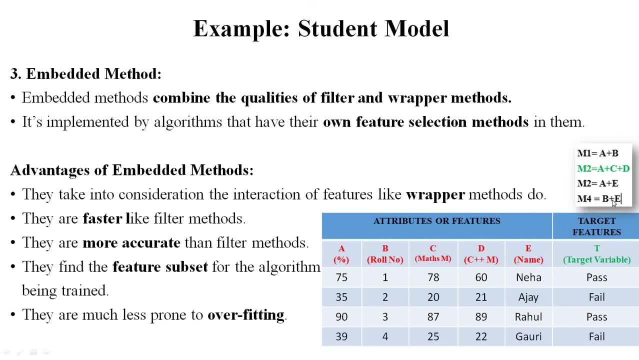 Okay So, embedded method. first make a model as like wrapper method. Okay, So here is a model like M1, M2, M3 and M4.. This is a wrapper methods model that I have already explained in last slides. 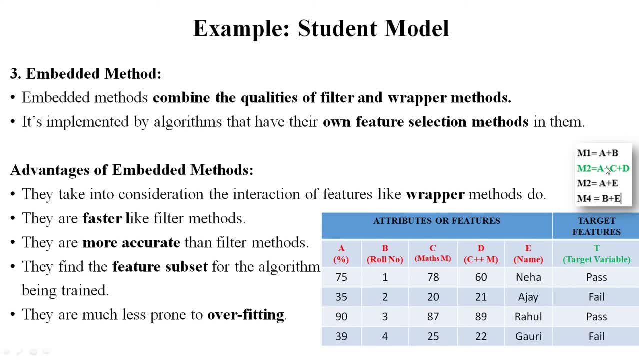 Right Now embedded method, identify which is the best model. The best model is A plus C plus D, Right. So from that features. again, they identify which is the best feature, like filter method. So from that, A plus C plus D, which is the best feature. 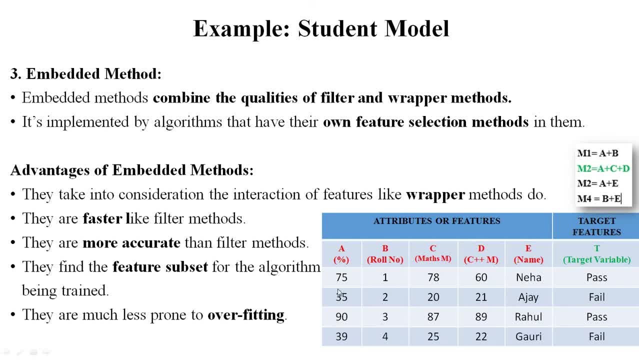 The best feature is A, that is percentage Right. So this is called as embedded method. It is implemented by the algorithms have their own feature selection methods. So the advantages of embedded method is they take the consideration to interact the features like wrapper methods. 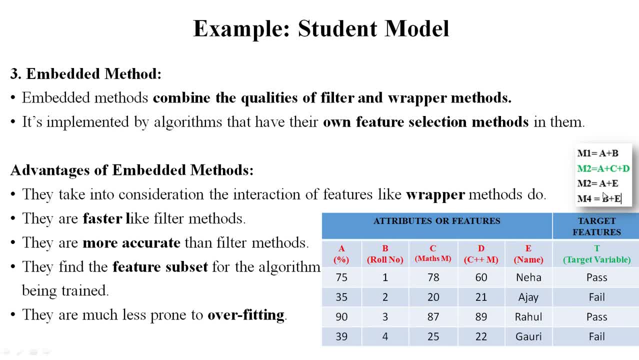 Okay. They first wrap the features and they identify the one of the best features from that particular data set. So this is the more faster method as compared to filter and wrapper method and the result of embedded method is more accurate as compared to other filter method. 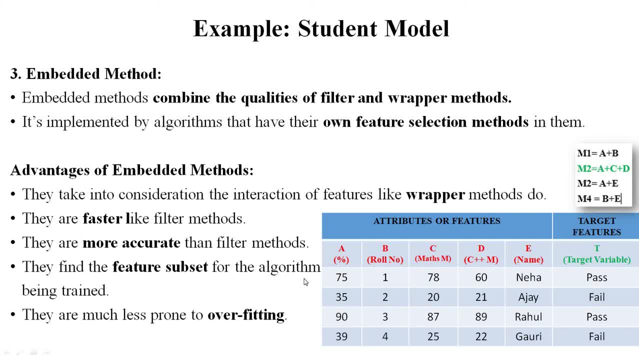 So they find out the feature subset and optimal features For each and every algorithms. that being trained Right And this algorithm are much less prone to overfitting means less number of errors are generated in this model. So this is the concept of embedded model. 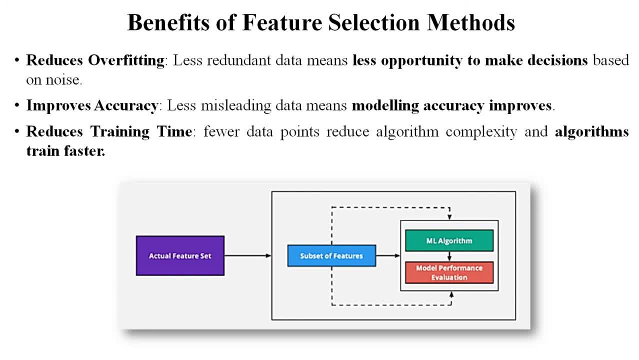 Now, what is the benefits of feature selection method? We have learned the three methods, like filter method, wrapper method and embedded method. So what are the benefits of feature selection method? See here in this diagram. So in this diagram, this is your actual feature set. 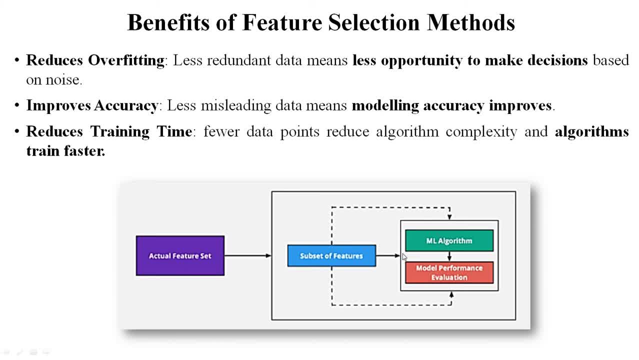 Okay, Means suppose there are 10 number of features. You have to identify the relevant features by using those method, So this is called a subset of features. Okay, And this relevant features are used by the machine learning algorithm to evaluate, to identify the performance of the model. 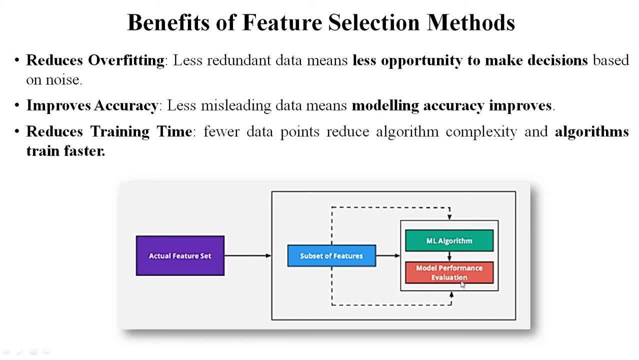 Right. So by using this relevant features, the particular model generate more accurate result. So the benefits of feature selection: first one is a reduce overfitting Means. you should reduce the irrelevant features, you should reduce all the duplicate data, So less opportunity to make a decision based on noise. 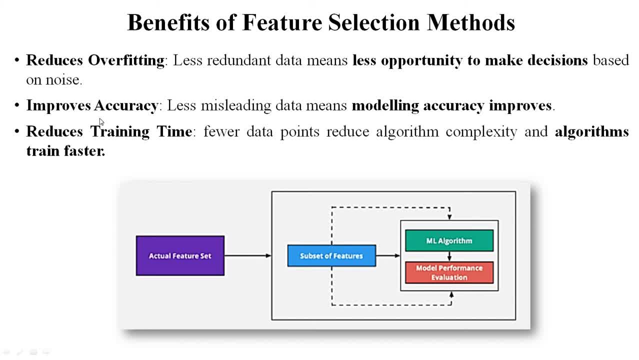 So this is the benefit of feature selection. The next one is improve accuracy. Your model accuracy will be improved by using relevant features for training purpose. Now, next one is reduce training time, Because fewer data points reduce algorithm complexity and algorithms train faster. 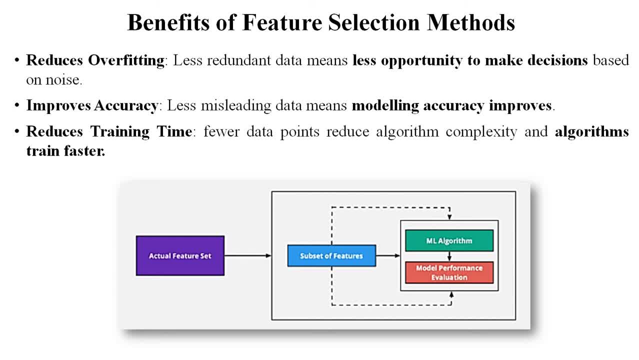 Because we have reduced all the noise, reduce all the duplicates, Data Right, We use only relevant features, So the training time is also improved. So these are the benefits of feature selection methods. Now the next concept is feature extraction. 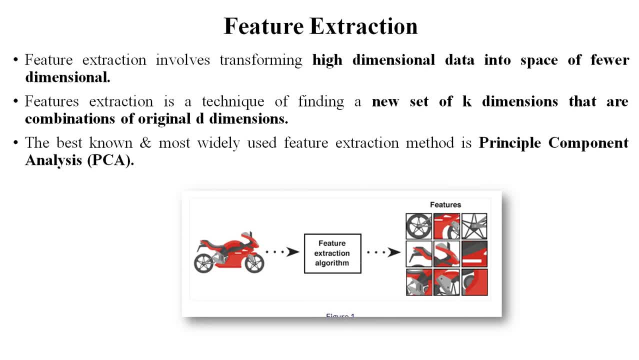 So in last slides we just select the particular feature Right. So for training purpose we have to extract those features and send to the those features to the particular machine as a input Right For training purpose. So feature extraction, This concept is called as to convert high dimensional data space into the lower dimensional.